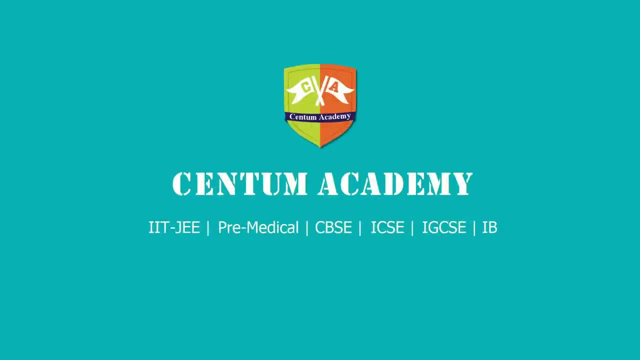 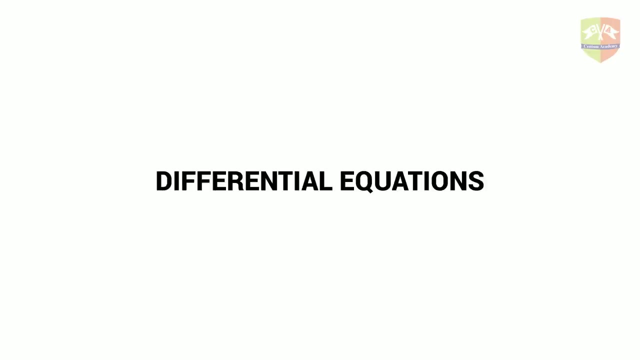 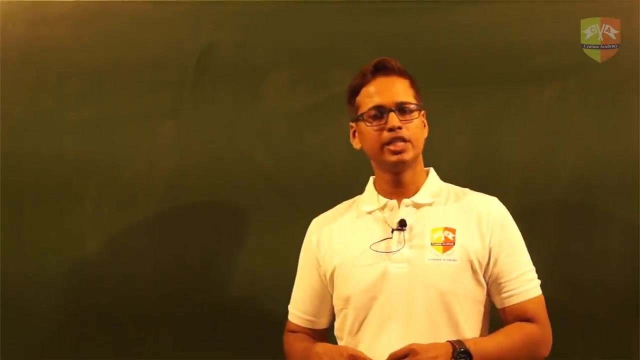 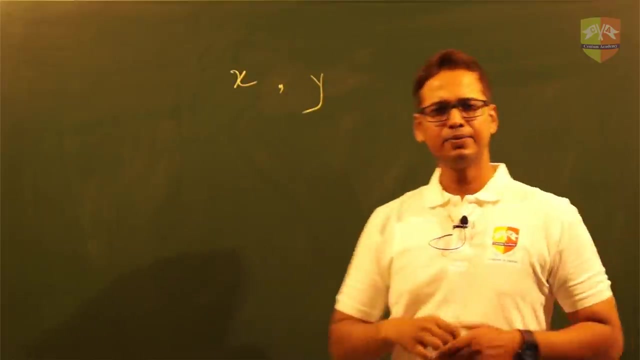 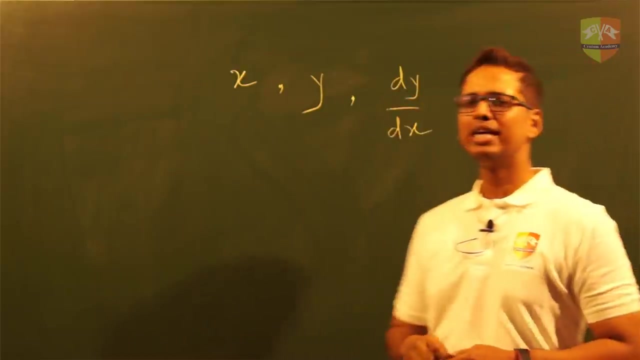 Alright, so what is a differential equation? A differential equation is basically an equation which involves the independent variable x, the dependent variable y and the differential of the dependent variable with respect to the independent variable, that is, dy by dx and dy by dx can be in. 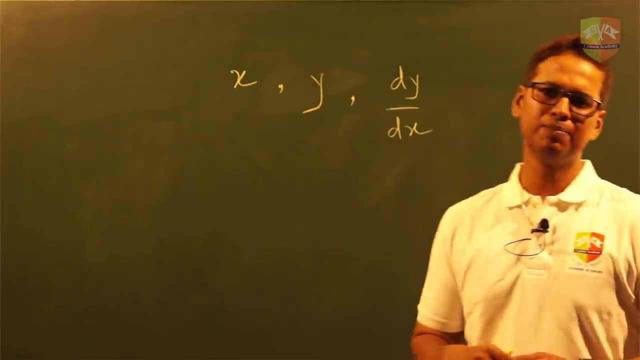 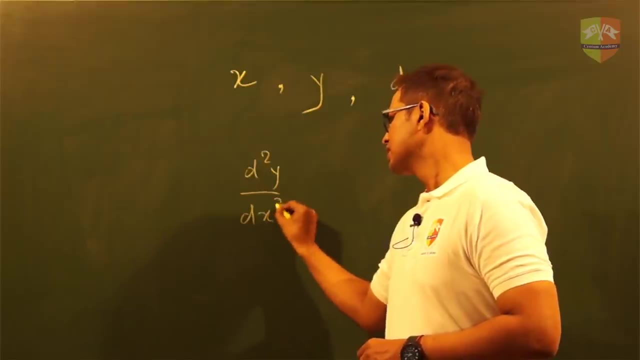 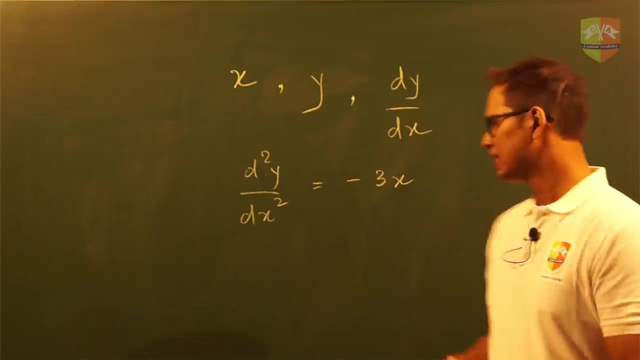 various orders. right To give you an example of a typical differential equation, something like: d2y by dx square equal to minus 3x. okay, So basically this is a differential equation. We can have a y as well here, okay, So basically this is a differential equation which involves: 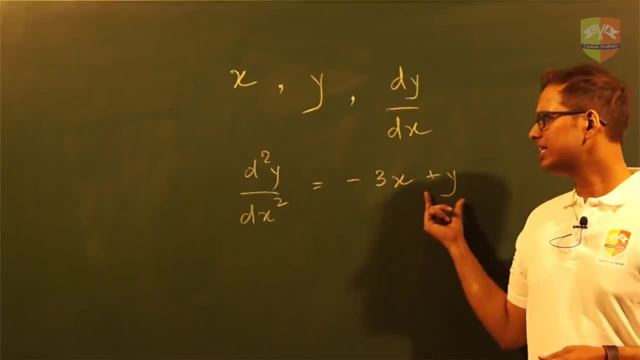 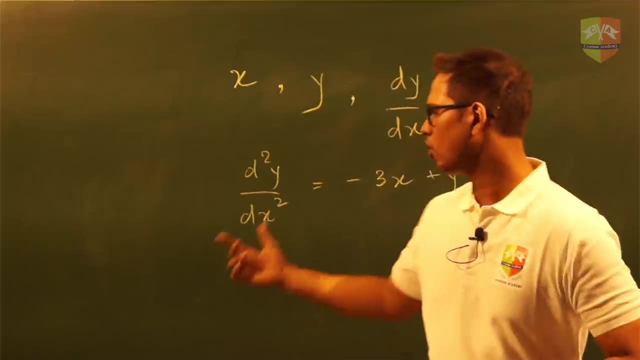 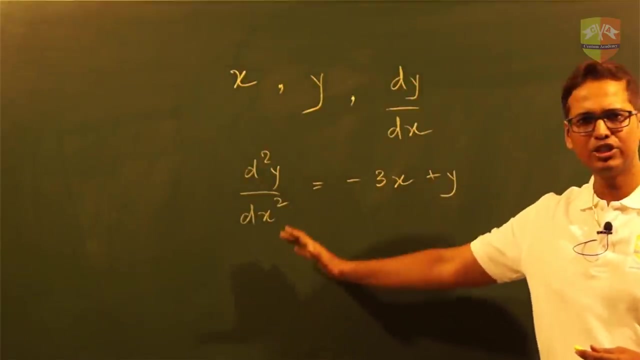 a independent variable, dependent variable and a particular order. There may be various orders of the differential coefficients involved. This is called a differential coefficient of second order, So any kind of equation which involves a relation or an equation involving x, y and various. 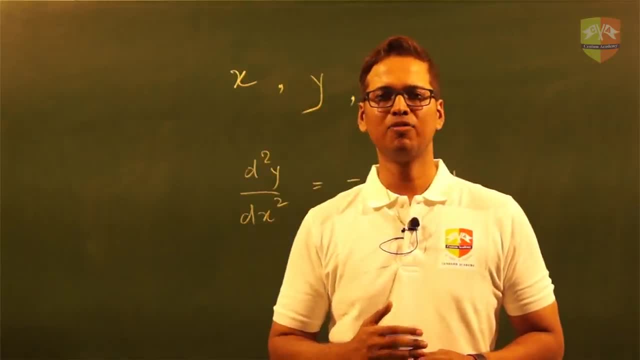 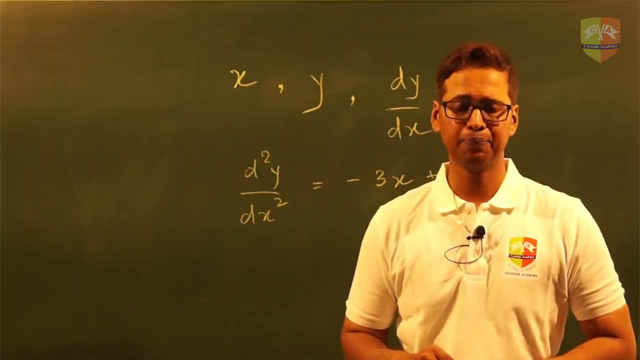 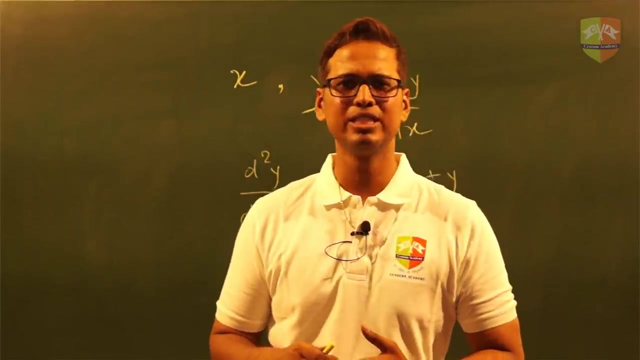 orders of the differential coefficient of y with respect to x and, of course, constants can be. there is called a differential equation. right The use of differential equation? like it's tremendous If you're talking about physics. you use this in the simple harmonic motion. right, You can use. 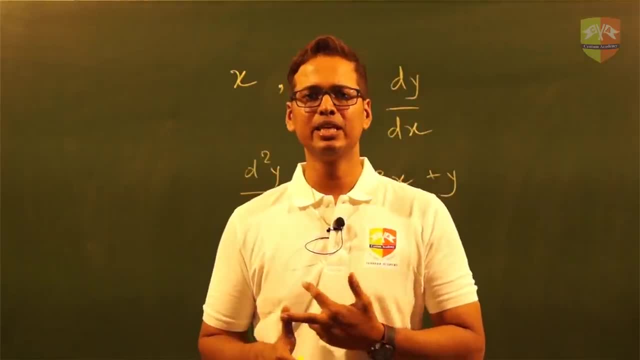 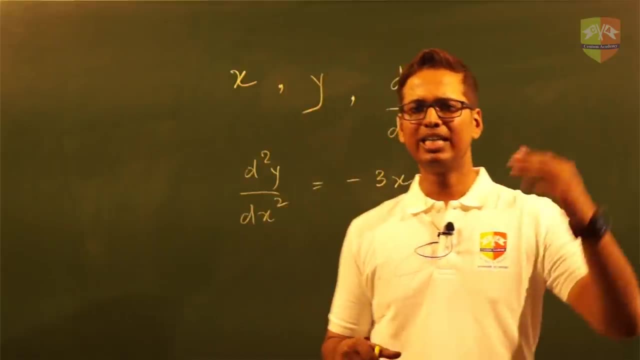 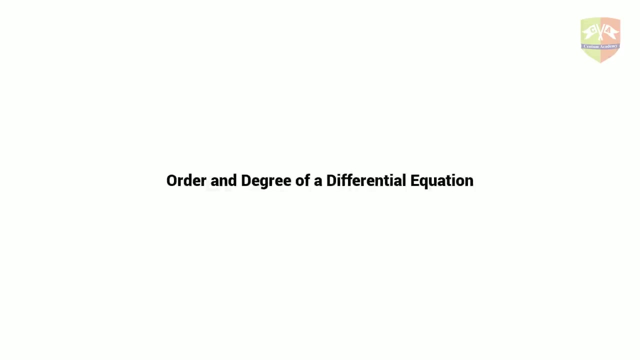 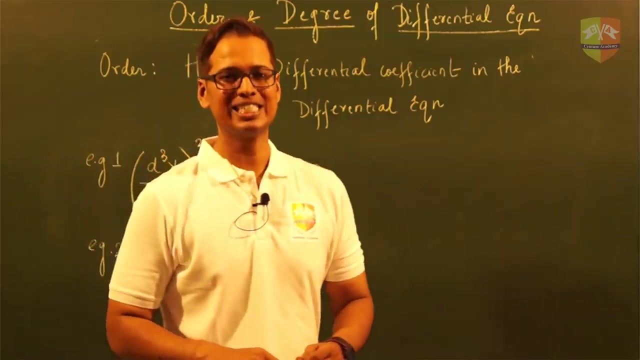 the RC circuits. You can use this in chemical kinetics. In the last part of the chapter, when we're doing the application of differential equations, will take a lot of example where we'll show you the physical relevance of differential equations for you. All right, Students know, let's talk about the order and degree of the differential equation. the order of the differential equation is called the. 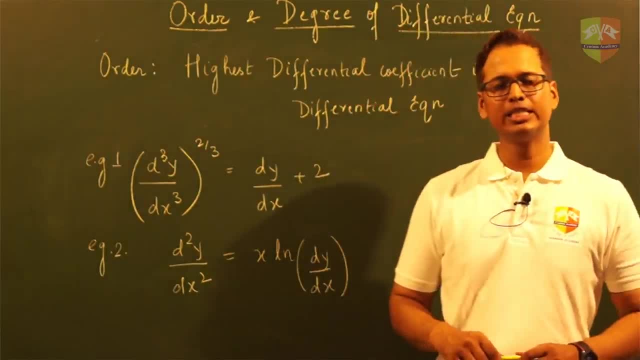 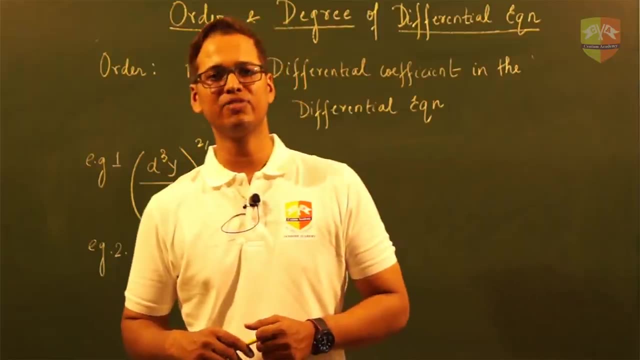 How to make a differential equation for physical engineering. now, order of the differential equation is called differential equation for research, and its names is nothing but the highest differential coefficient of y with respect to x which occurs in that differential equation. To give you some examples of what I mean when I say: 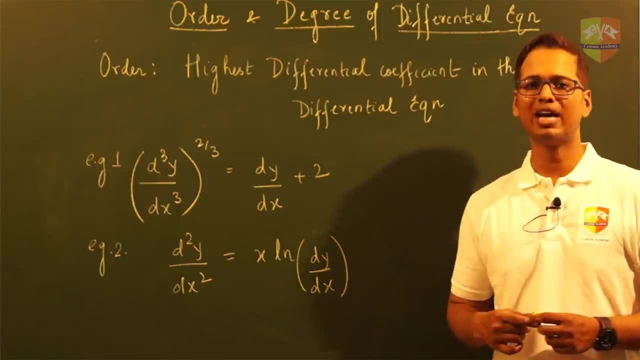 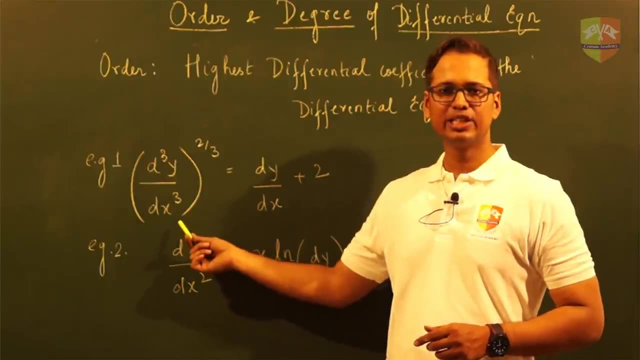 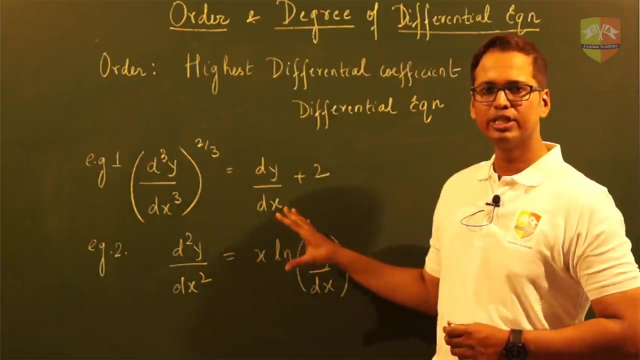 highest differential coefficient of y with respect to x. let us take example number one. In this you can see we have d3y by dx cube raised to the power of 2 by 3, equal to dy by dx plus 2.. In this particular differential equation, you would realize that the highest differential 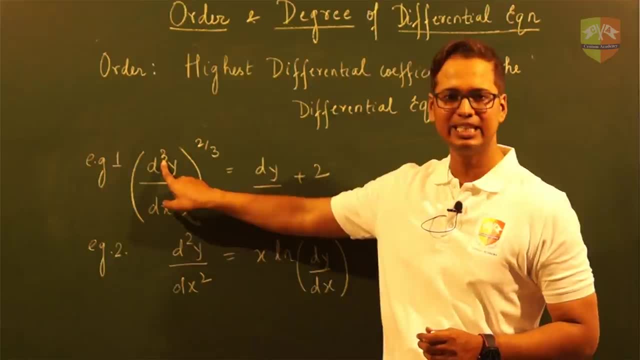 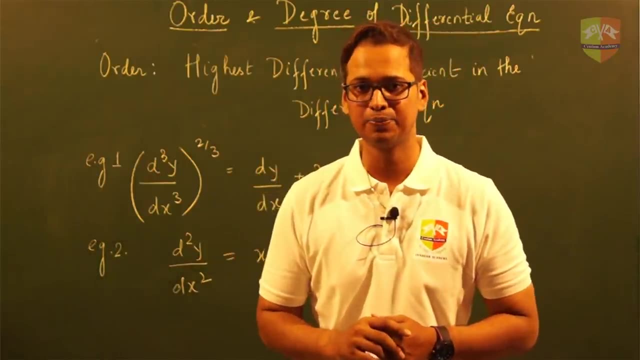 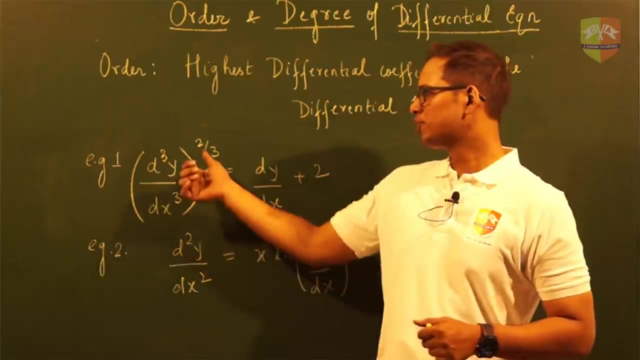 coefficient of y with respect to x is 3.. This means it has- y has been differentiated a maximum number of three times with respect to x. Please note: this power has no relevance while deciding the order of the differential equation, So please do not take into account that, since there is a 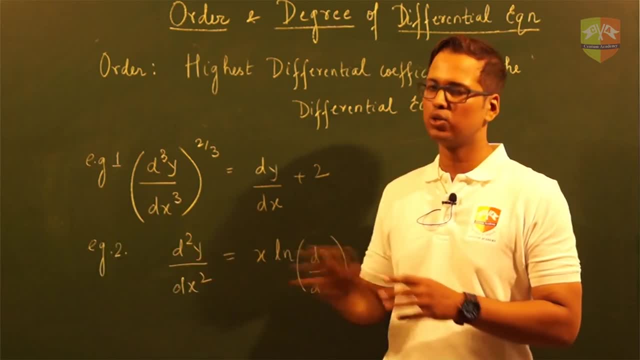 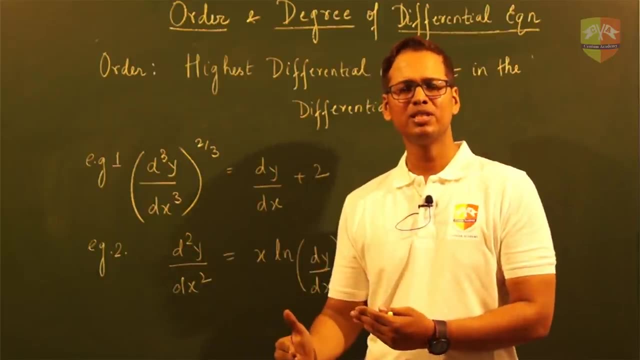 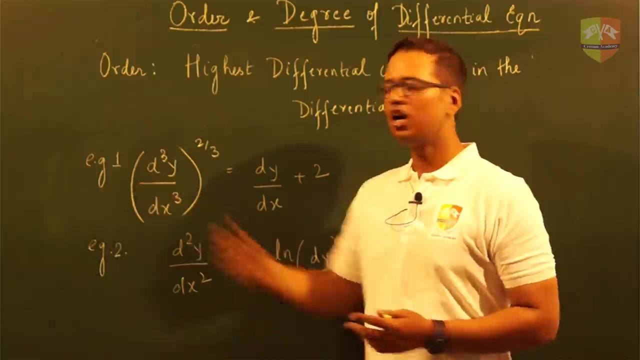 power of 2 by 3, it should become a d2y by dx square. No, that doesn't happen. In this case we say: the order is nothing but the maximum number of times of the derivative of y that has happened with respect to x in that equation. So this is a order 3 differential. 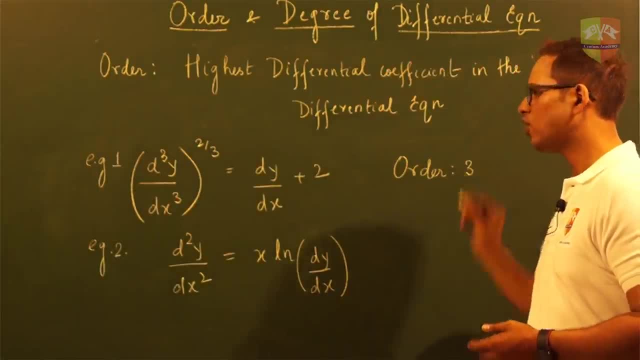 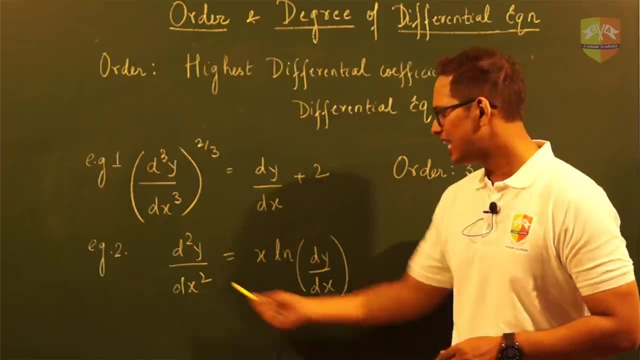 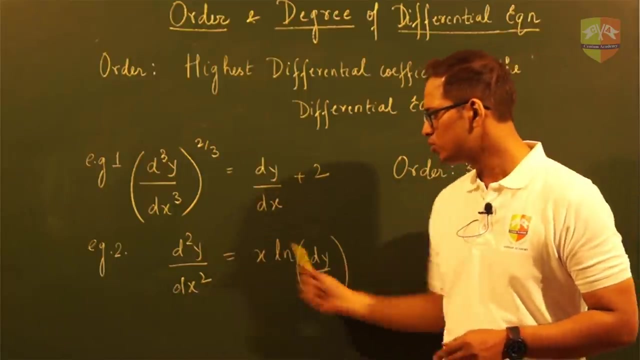 equation. So we say this is a differential equation of order 3.. Let's take example number 2. You can guess, you can take a call. you can see that dy by dx, d2y by dx square is equal to x, ln, dy, dx. So out of these two the highest order is given by this term, because here y has been. 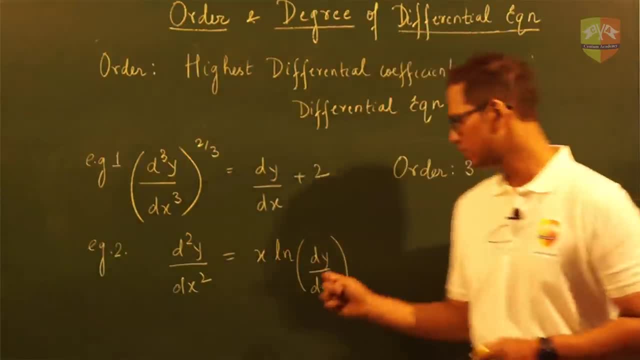 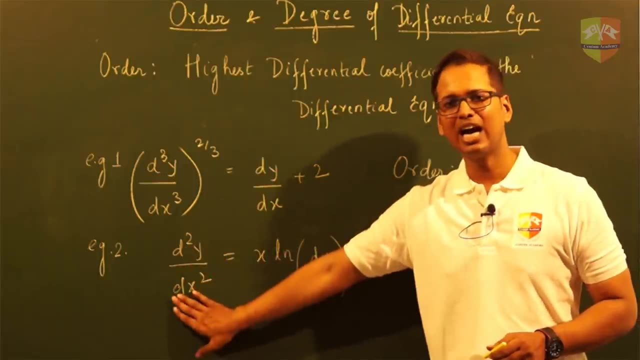 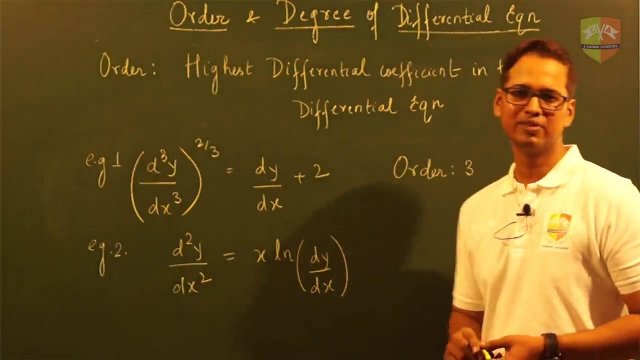 differentiated twice with respect to x, Whereas in this expression y has already been differentiated once. So out of the two, since this is the higher, we say that the order of this differential equation will be nothing but 2, because 2 times derivative has occurred here. So this is a differential. 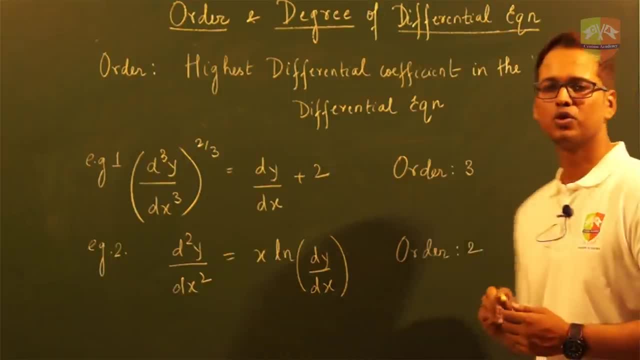 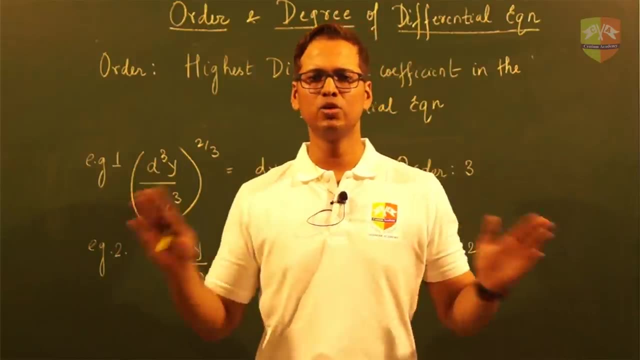 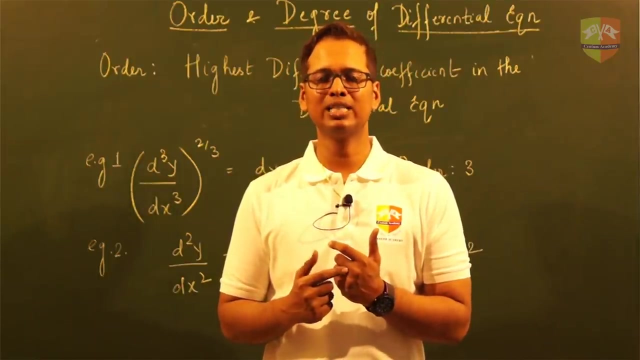 equation of order 2.. Again, repeating a very, very useful information. When we are deciding on the order, we just look into the entire expression and pick out that term where the derivative of y with respect to x has happened maximum number of times. That decides the order of the differential equation. 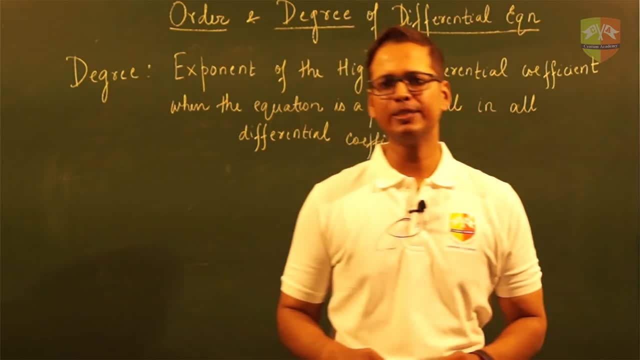 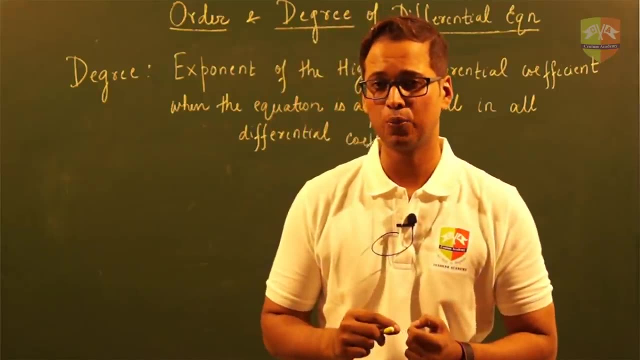 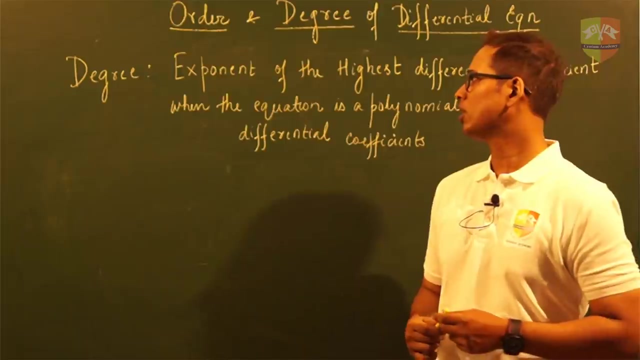 All right, student. now let us understand degree of the differential equation. Now, this aspect of degree is slightly critical, So you have to be very, very attentive while listening to whatever I say. now, The degree of a differential equation. as I have already written on the board, You can, we can read this, you know along. It's the exponent of the highest. 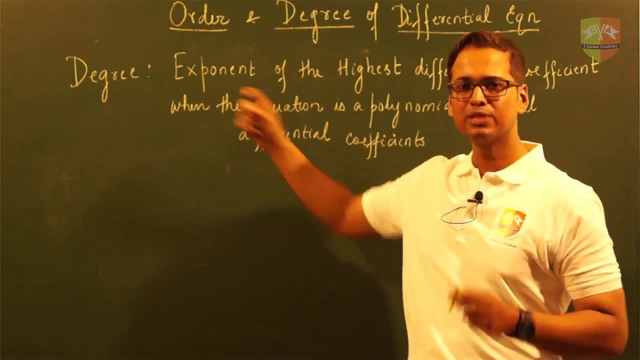 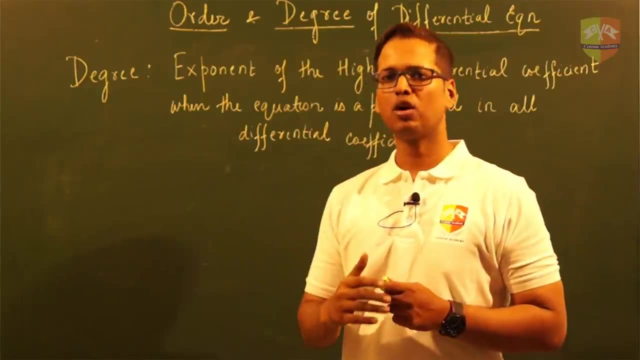 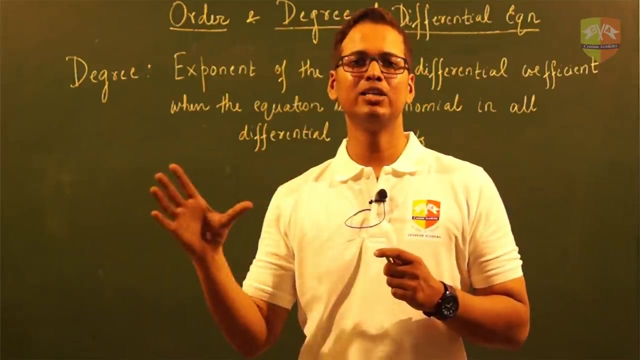 differential coefficient. What is the exponent? Exponent means the power. It's the power of the highest differential coefficient. Now, in the previous video, we had talked about the order of the differential equation, where I had taught you how to identify the highest differential coefficient. That means what is the maximum number of times the derivative of y has. 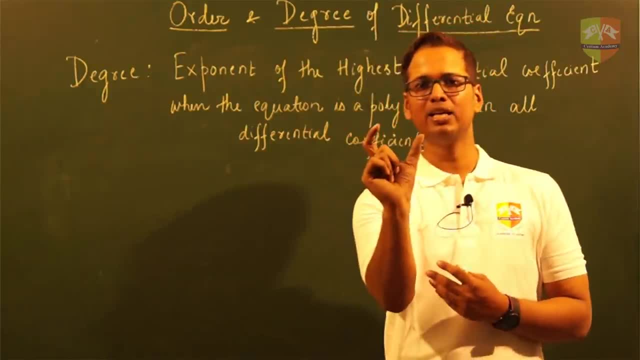 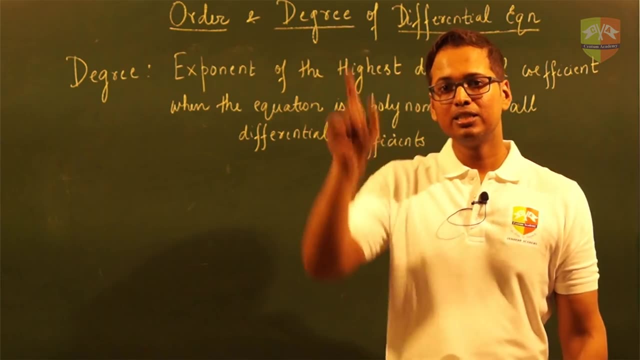 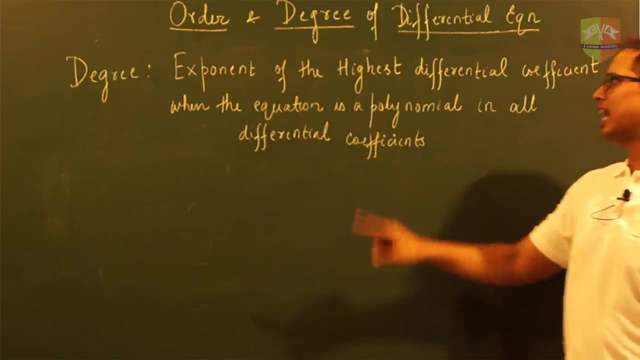 occurred with respect to x. So, once you have identified the highest differential coefficient, which is nothing but which decides the order of the differential equation, the power of that term, that is the exponent of that term, when that differential equation has been expressed in the form of a polynomial, 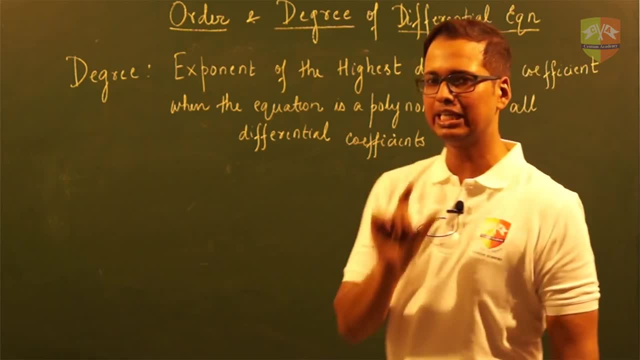 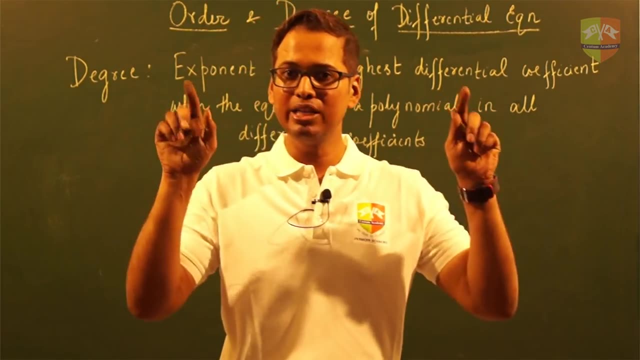 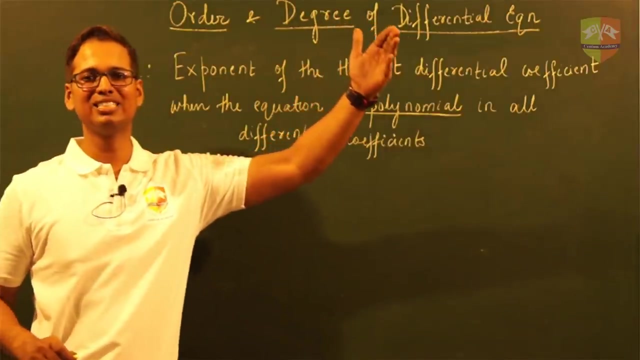 in all the differential coefficients. Now, this is slightly critical. What do I mean when I say when the differential equation has been expressed as a polynomial- the word polynomial- in all the differential coefficient? Now, let us go back to our class 10th. What do we understand from a polynomial? Now, if you recall a polynomial, 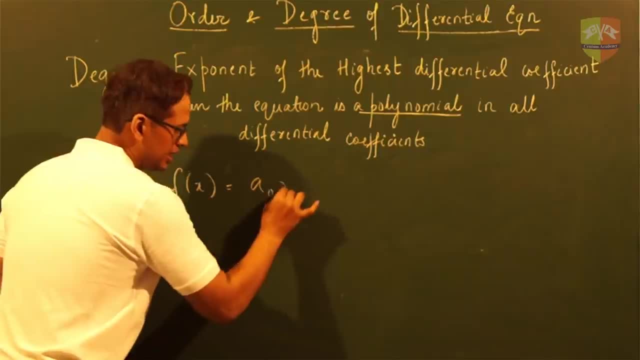 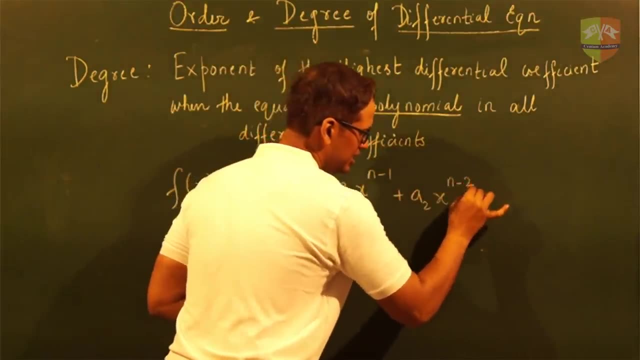 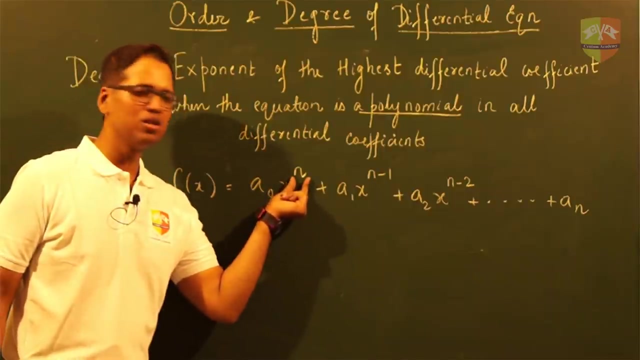 function is something where you have terms like this, right? So we have terms of the state of the number of factors, strings all around the whole square root of the number of factors, strings in the number of the public sector, or something like that, right? So what is the power of that 0?? That is a. 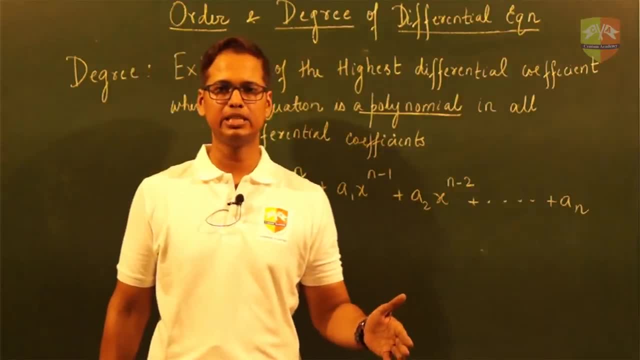 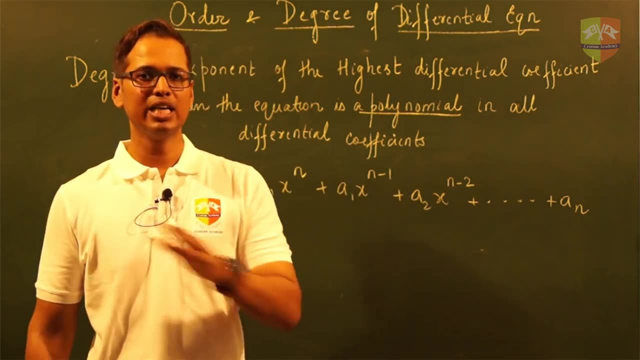 function of the number of factors exchange over the giri sound, meaning the number of factors which actually 作 as a function on a polynomial- and again, this is for the less than escribblers who are least good customers of noscarg ever moppedでしょう- and even numbers. 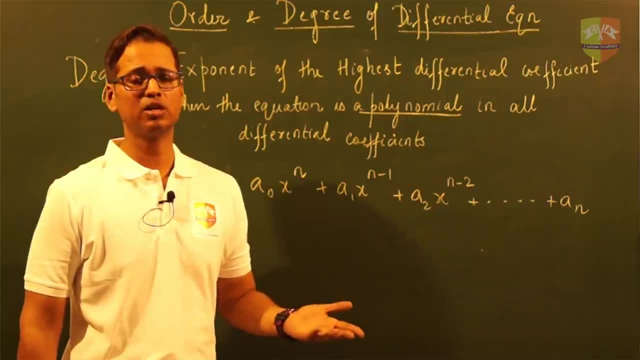 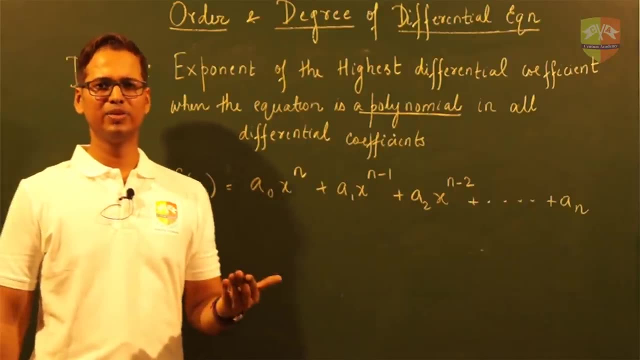 So you have a Kazakh: reduces 그래도 좀. do you want using this, whether say must not be, they must not be in negative integers. in a similar way, when your differential equation has been expressed in such a way that all the differential coefficients, no matter whatever, 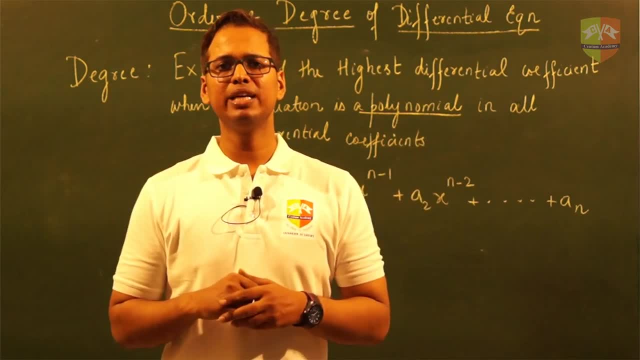 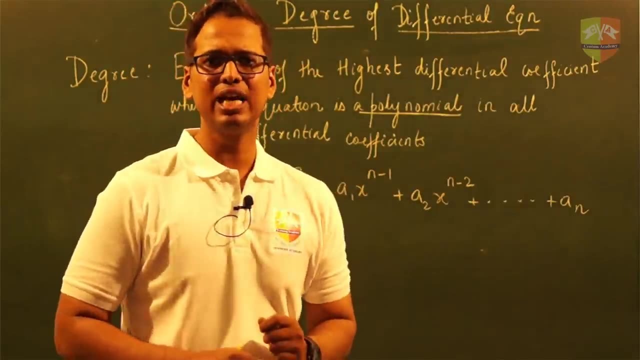 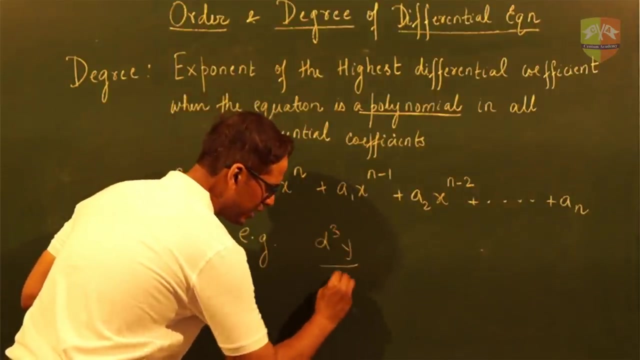 order. they are right. if their power has been made whole numbers, then only we can decide on the degree of the differential equation. let me show you with the help of an example. let's say i have a differential equation like this: d3, d3, y by dx, cube whole to the power of 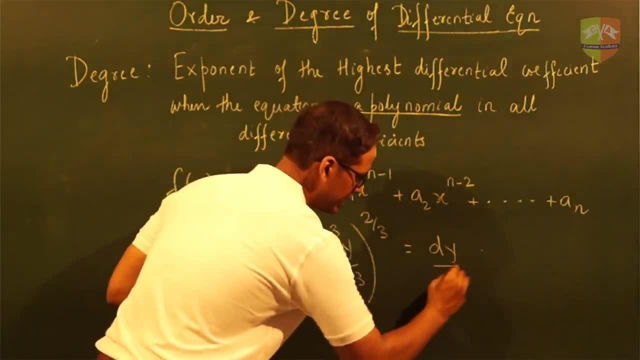 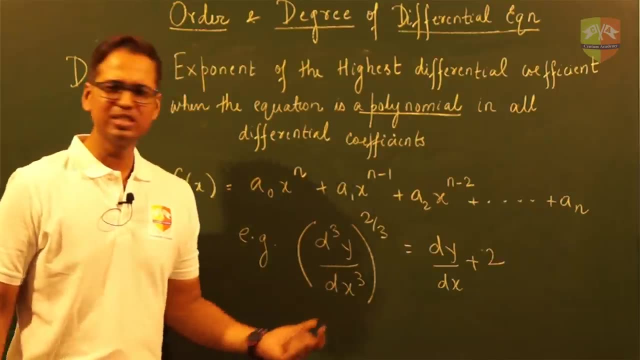 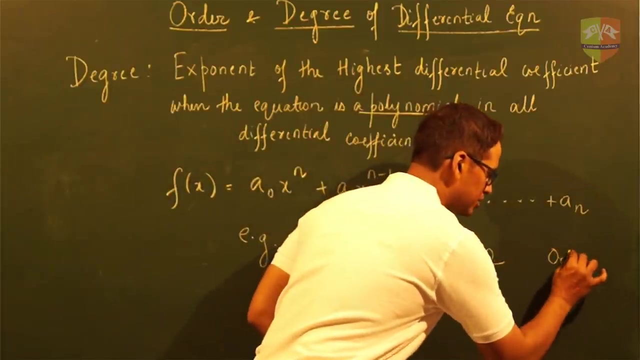 2 by 3, equal to dy by dx plus 2. okay, i've taken a very similar example in the previous video. also, the order of this differential equation is what? it's 3, right, this decides the order. so it is an order 3 differential equation, so order 3. so there is no doubt about the order. 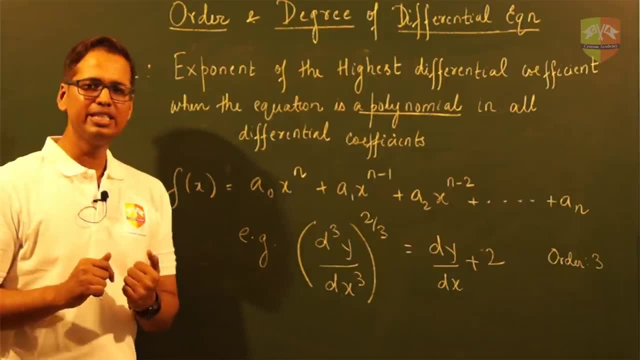 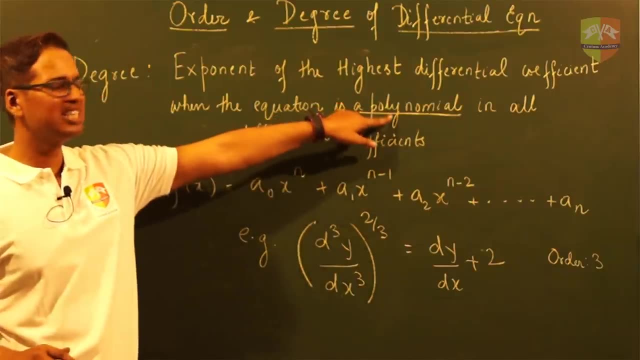 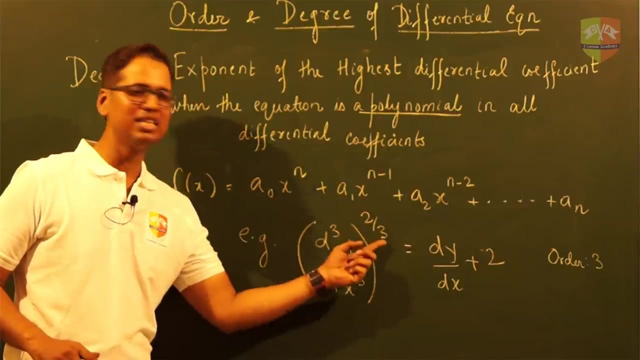 so there is no doubt about the order. so there is no doubt about the order, but wait a minute. when i'm deciding about the degree, have i expressed this in a polynomial of the differential coefficients? no, we have not expressed in the polynomial of differential coefficients, because the power on this differential coefficient is 2 by 3, which is not. 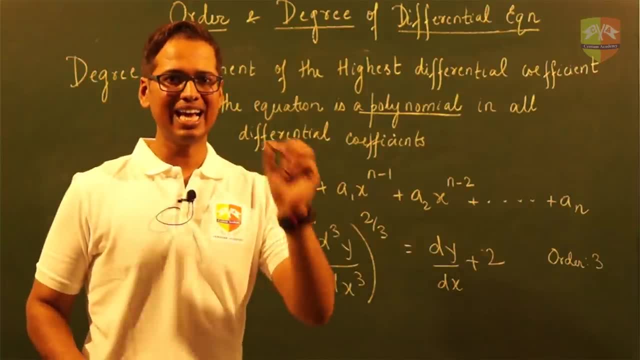 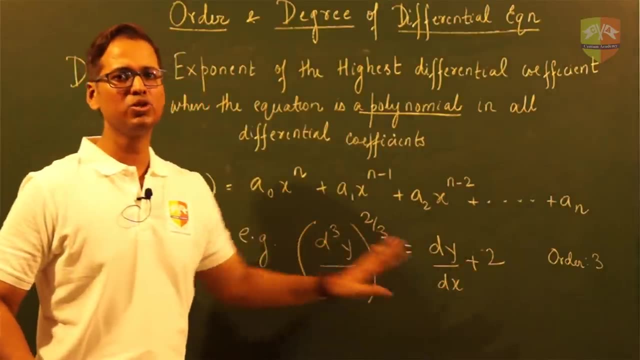 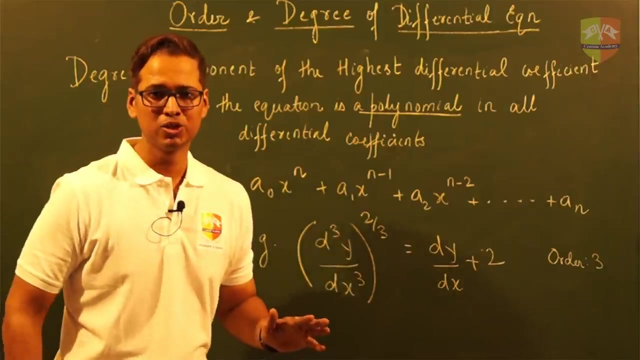 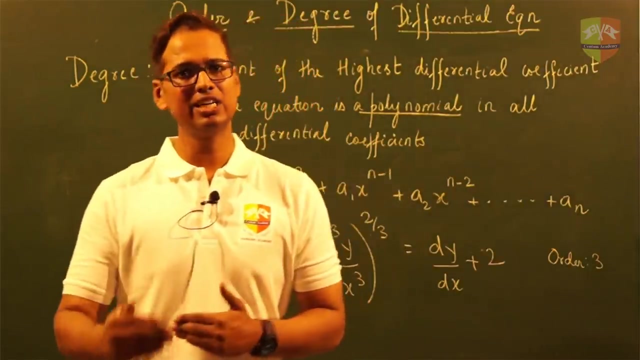 allowed in a polynomial. so in a polynomial, x should not have a fractional power. in a similar way, this differential coefficients involved in this expression should not be allowed in a polynomial. so thisUp kami na you have is equal to m by m divided by m x. outside, this is called a. 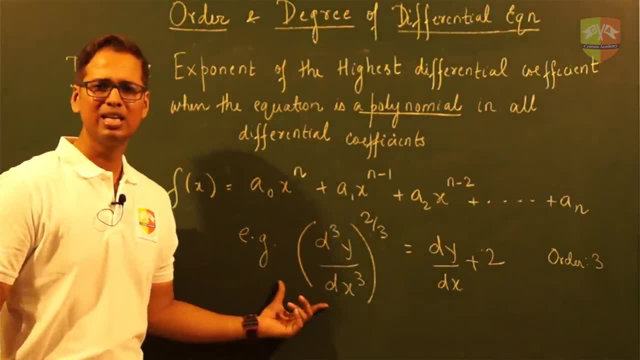 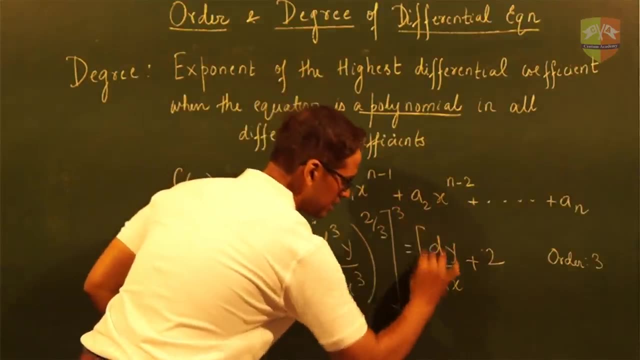 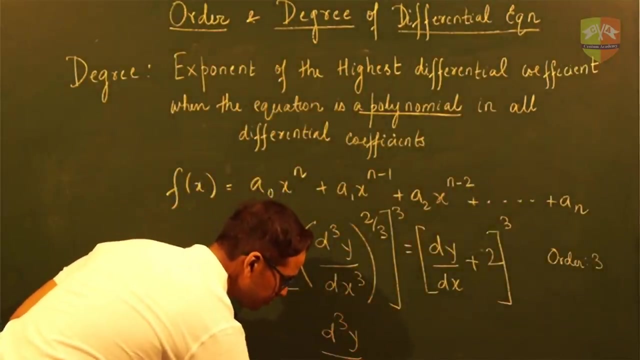 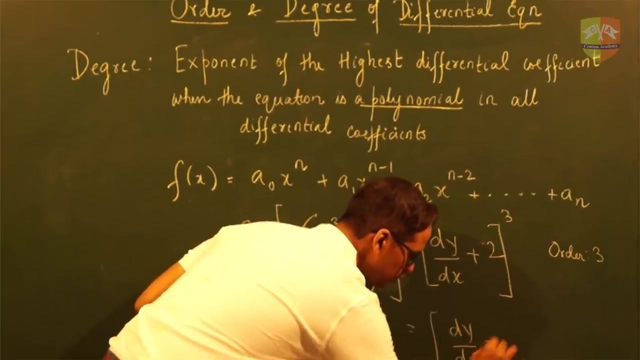 Grasshopper. now let's break it down and just, we are going to have a part of the interval, any part. one, I am told, is 0 to half, away from 0…. 3y by dx- cube, whole square equal to dy by dx plus 2, the whole cube now having. 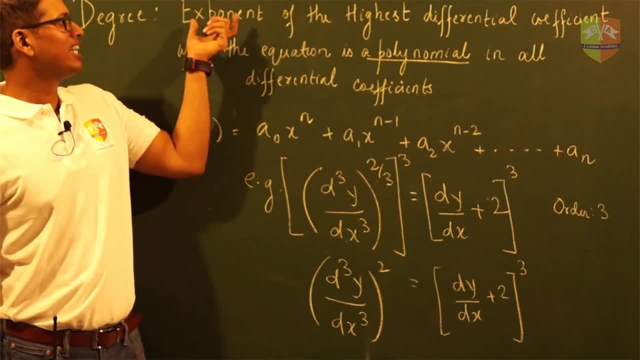 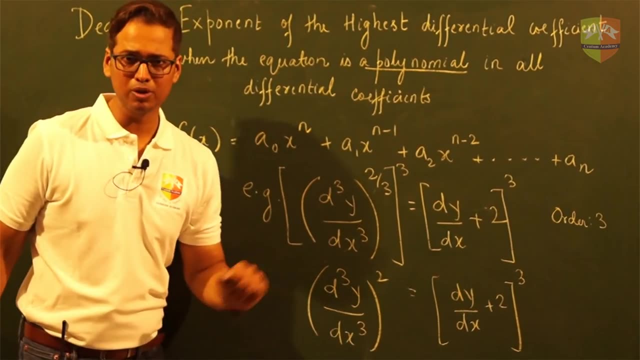 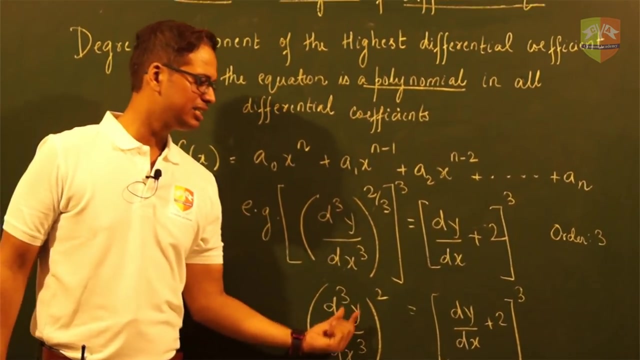 done this. now what is the highest, or exponent of, the highest differential coefficient? the highest differential coefficient is d, 3y by dx cube. no doubt about that. the exponent of that is 2, right. so, having converted it to a polynomial, the highest power of, or the power of the highest differential. 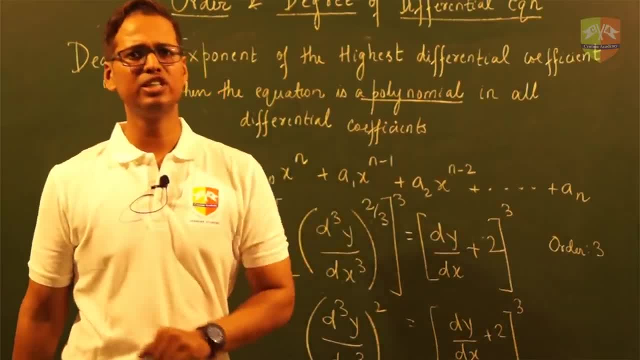 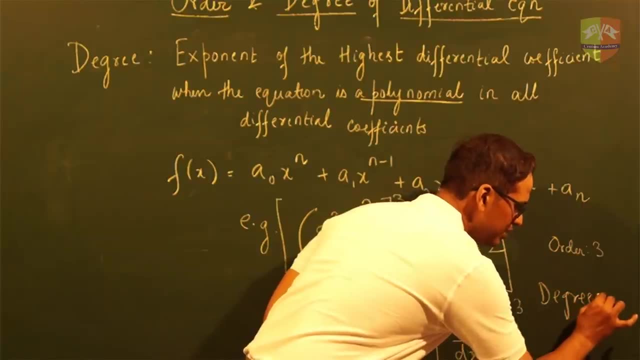 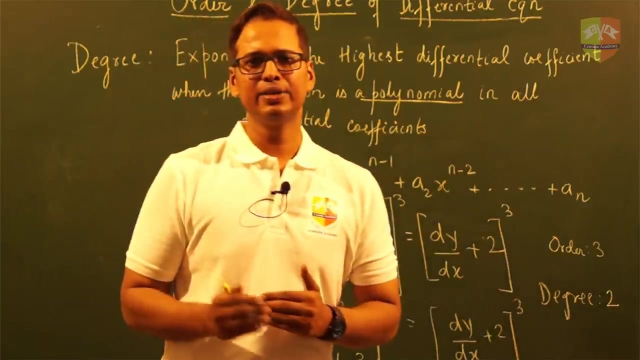 coefficient is 2, so hence this differential equation will have a degree of 2. so this will be differential equation whose degree will be equal to 2. right, hope it makes sense to you. so while finding the degree, two things you must keep into account: what is the coefficient or what is the exponent of? 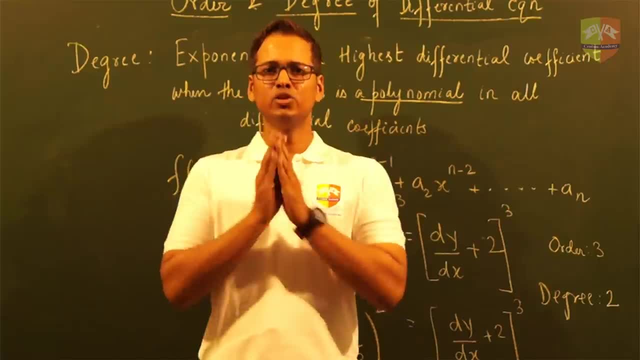 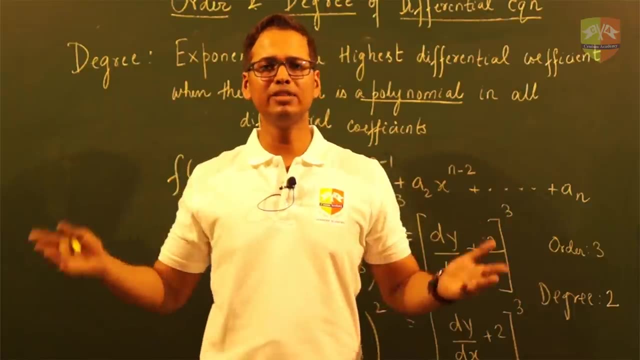 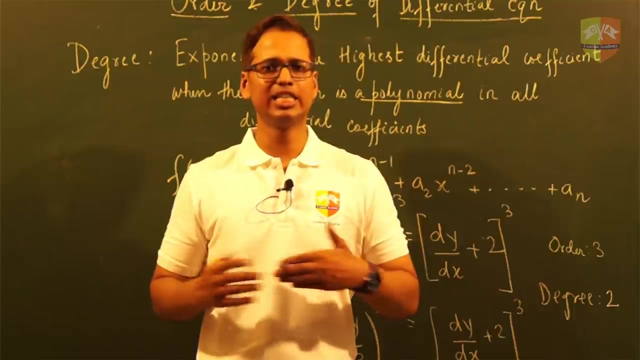 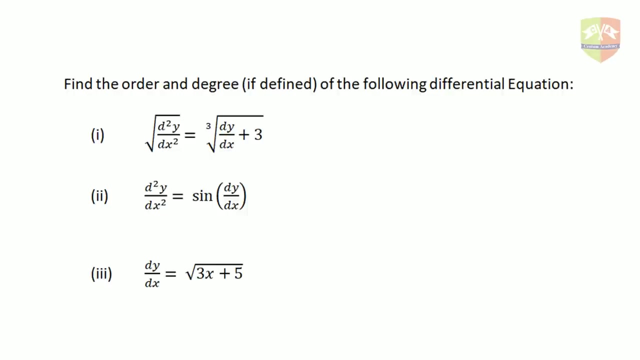 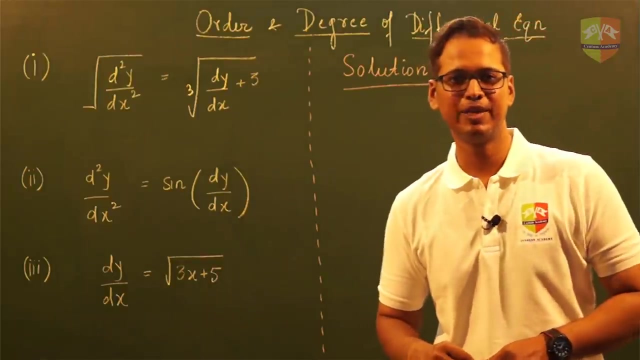 the order and you must convert that differential equation into a polynomial for a polynomial form in all the differential coefficients. if it is not, degree cannot be found out. right, we say: degree cannot exist. a degree does not exist for that particular differential equation. you all right, friends. now let us solve the questions which we just now displayed on. 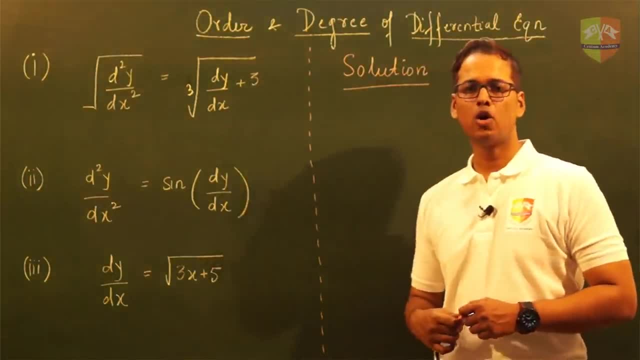 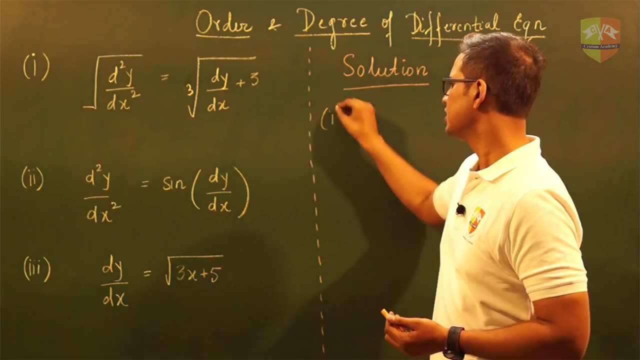 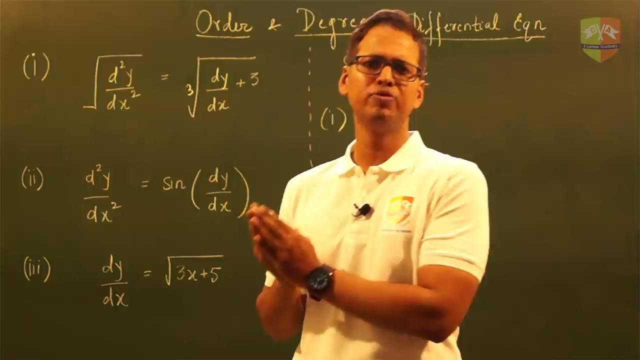 the screen. so we'll start with the first question. we need to find the order and degree of this differential equation. now, finding the order and degree of this differential equation is very simple. in order to find the order, we just see which is the highest differential coefficient of Y with respect to X. 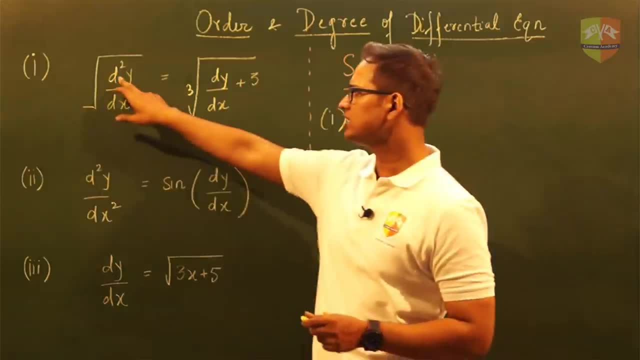 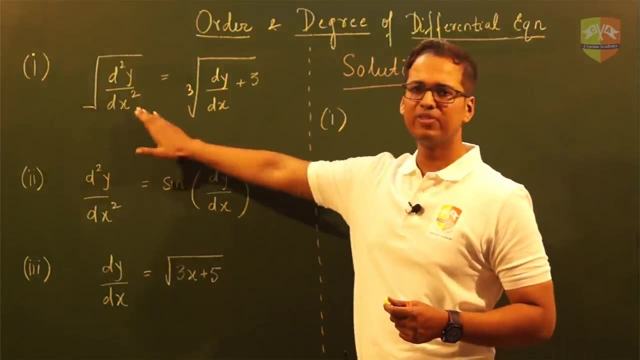 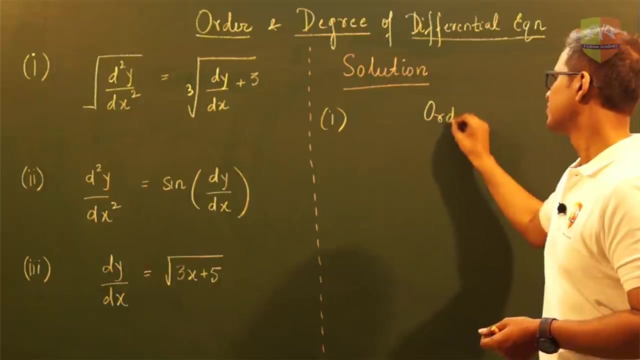 occurring in that differential equation, which clearly is this: d2y by dx squared term. right. so d2y by dx squared term is the highest differential coefficient of Y with respect to X in this video. hence, order becomes 2 right. so finding order doesn't take much time, you just have to identify. 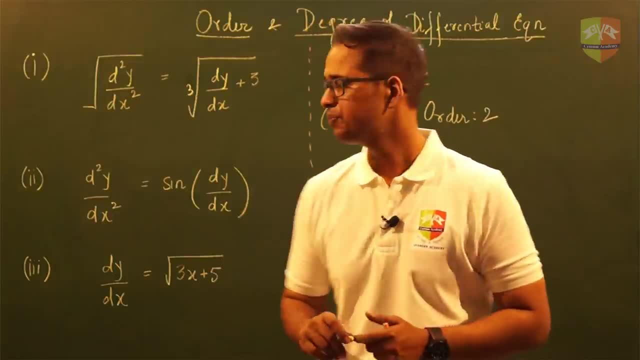 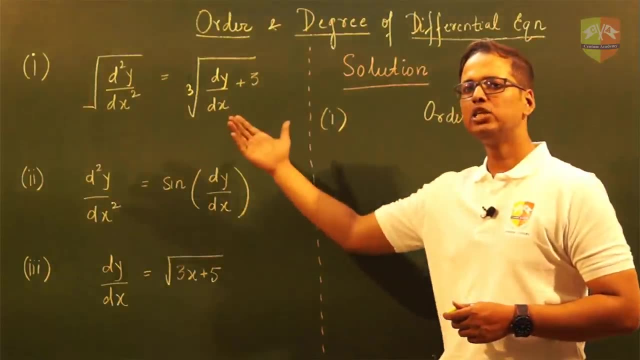 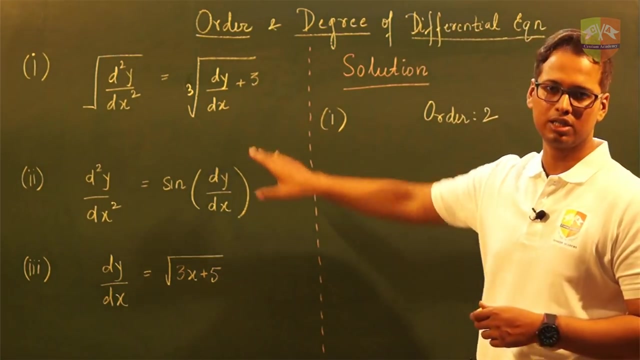 the highest differential coefficient. and your job is done right now. while finding the degree of this differential equation, we first need to convert this into a polynomial form in all the differential coefficients, right in the present stage it is not right because, if you see, the power of d2y by dx squared is half. 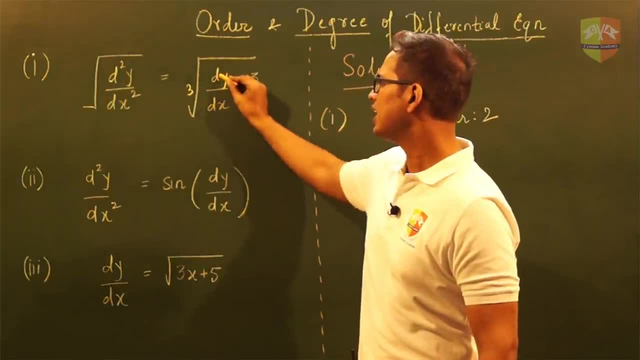 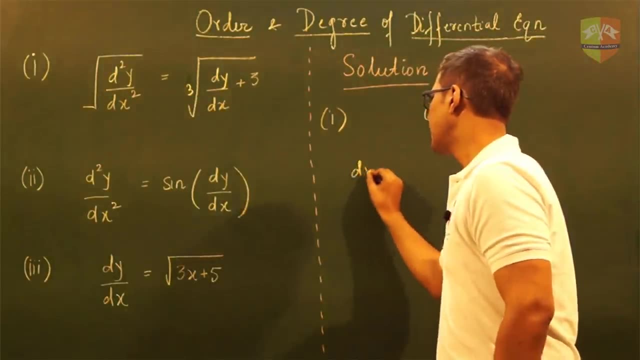 because it's under root and in this case we have dy by dx plus 3 whole subjected to the cube root power right. so if I have to write in terms of power, I can write this as d2y by dx squared to the power of half equal to dy by dx squared. 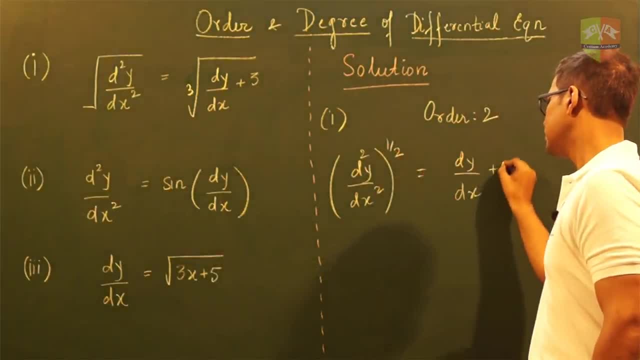 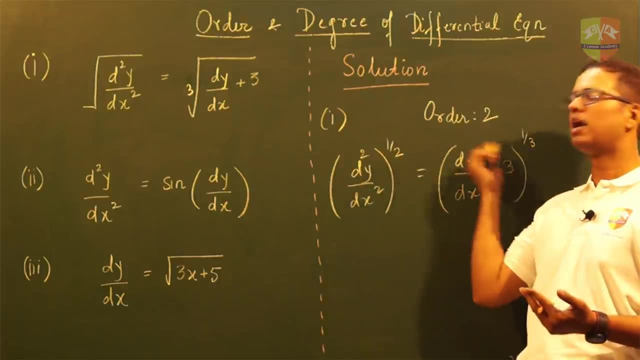 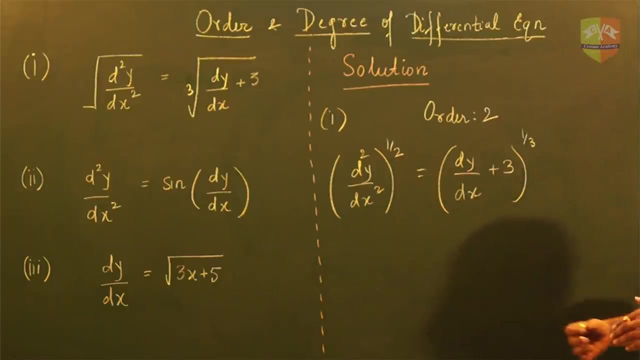 equal to dy by dx plus 3 whole, to the power of one-third right. and in a polynomial we cannot have these powers. so these powers are strict. no-no in polynomials right. so in order to convert it to a polynomial form, I need to apply some tricks. I need to first ensure 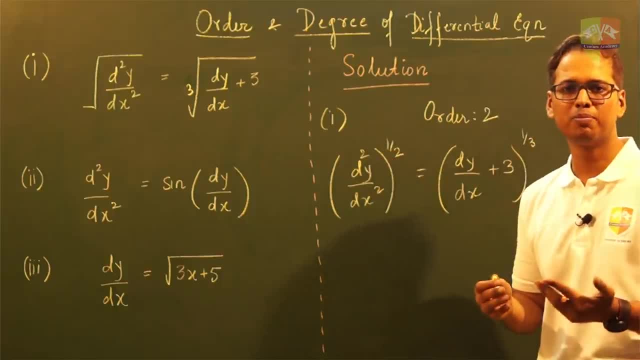 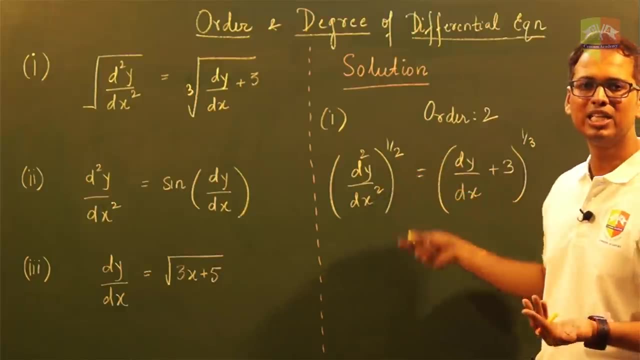 that I make these two numbers as whole number powers, and for that we need to multiply these powers by the lcd. Okay, So what I'm going to do is I'm going to take the lcd of 2 and 3. so lcd of 2 and 3, we all. 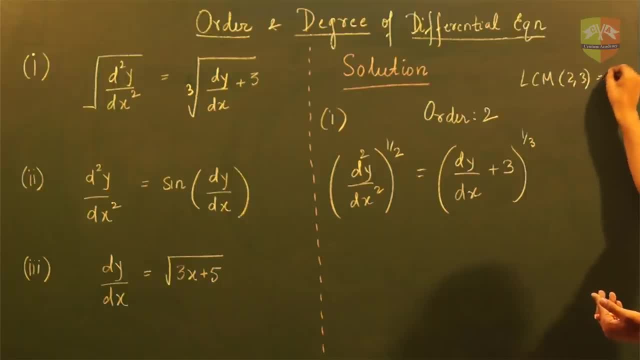 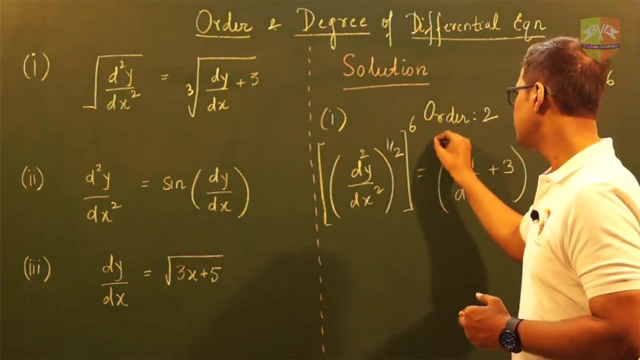 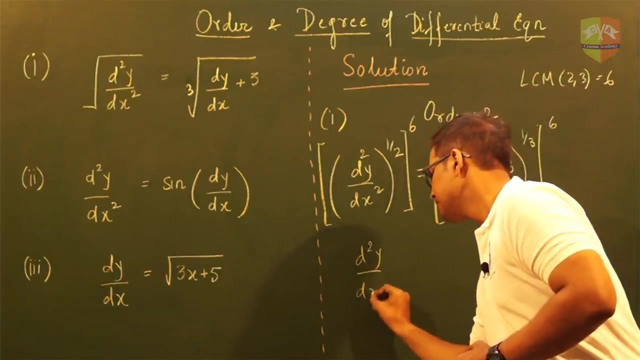 know lcd of 2 and 3 is 6. so what I'll do, I will subject both the side of the equation to the power of 6. so when I do to the power of 6 on both the sides of the equation, I would realize the left side becomes d2y by dx, squared whole to the power of 3, equal to dy by dx. 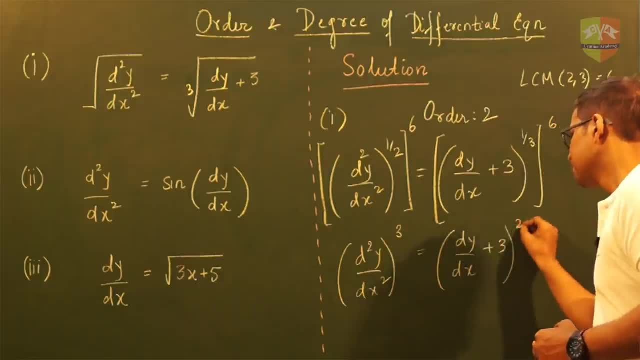 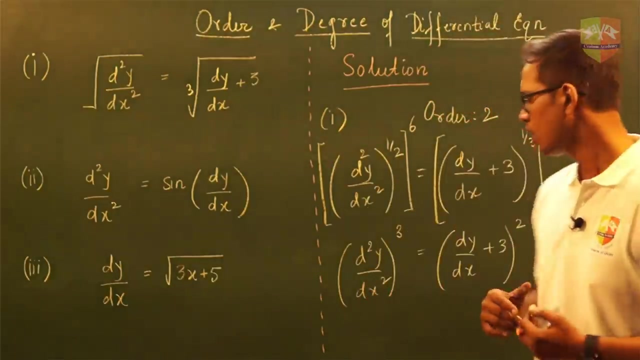 plus 3 whole, squared Right. having done this, I realize now each of the differential coefficients involved in this equation will be subjected to a whole number: power. that is what is meant by converting the differential equation in polynomial form. having done this, now I identify what is the 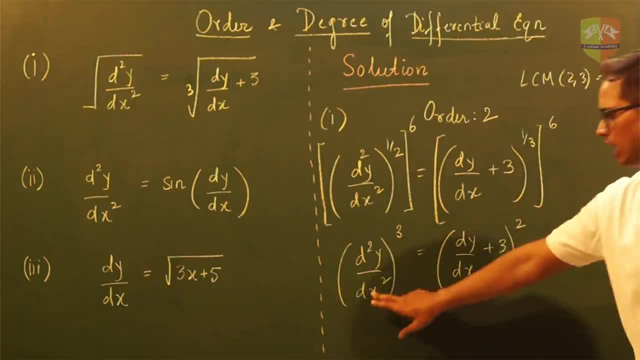 exponent of the highest differential coefficient. undoubtedly the highest differential coefficient is d2y by dx squared, The power of the exponent of this is 3.. So we say degree of this differential equation will be 3.. So this is an order 2, degree 3 differential equation. 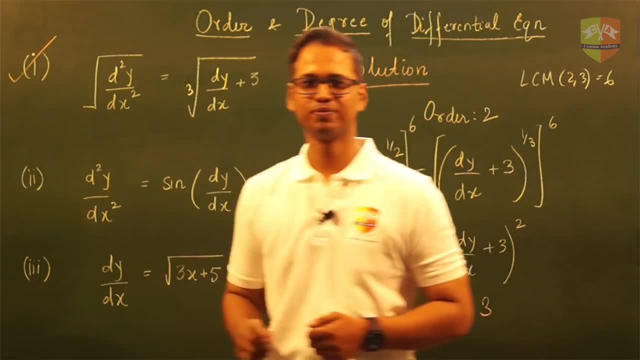 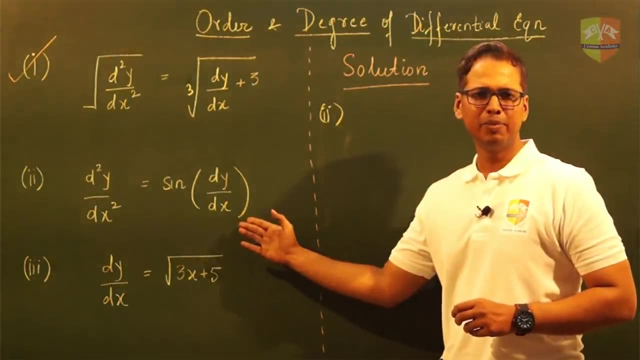 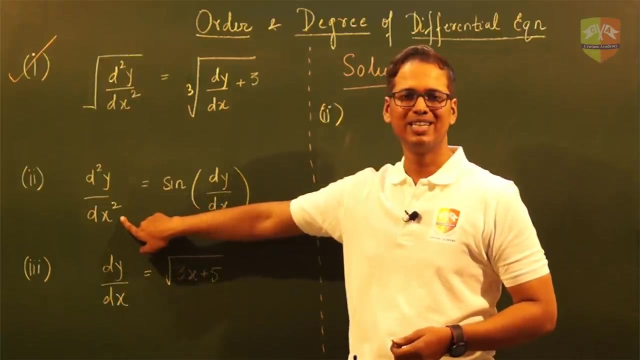 So this is how we solve question number 1.. All right, friends. coming to the second question now. finding the order again is a very simple task in this. we just have to identify the highest differential coefficient of y with respect to x. undoubtedly it is this term right: d2y by dx squared. 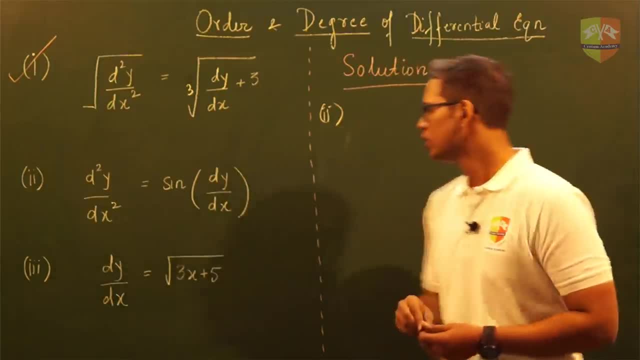 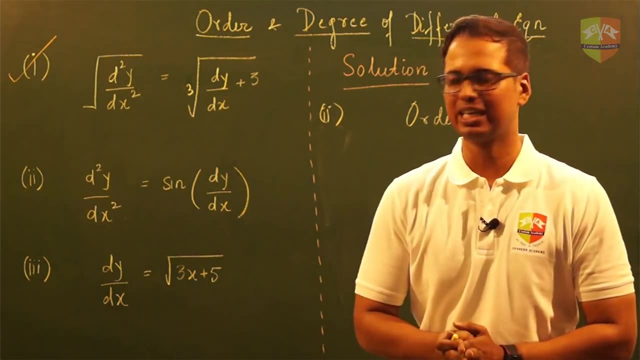 So d2y by dx squared. So d2y by dx squared corresponds to an order of 2.. So the order for this becomes 2: right finding order is the most easiest of both the activities. Now how to find the degree. now for degree, as I already discussed in the theory, we need: 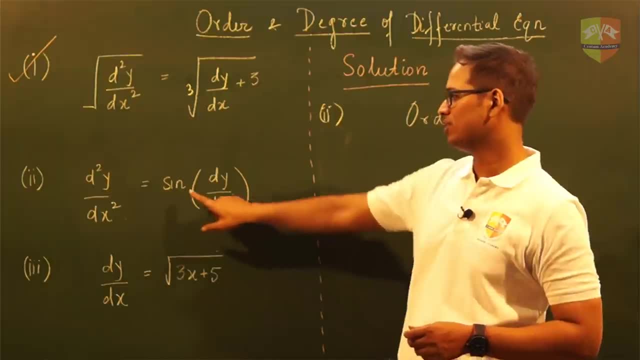 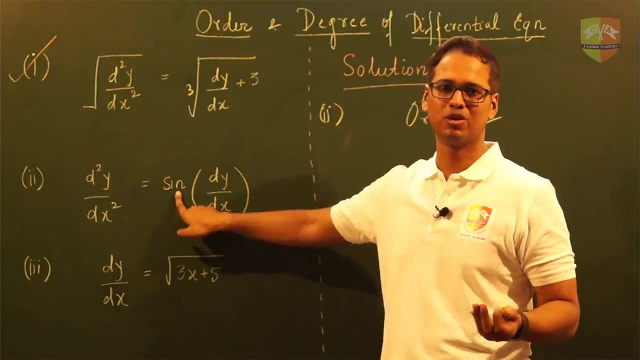 to convert this into a polynomial form. Now, this sign term here creates a problem, right? have you seen any polynomial having a sign term in it? No, of course not. A polynomial only has different powers of x. So this is a polynomial. So this is a polynomial. 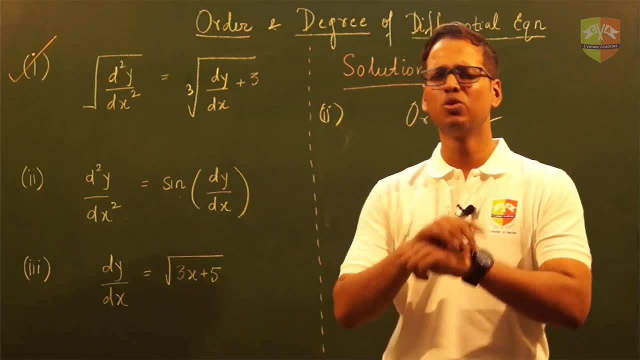 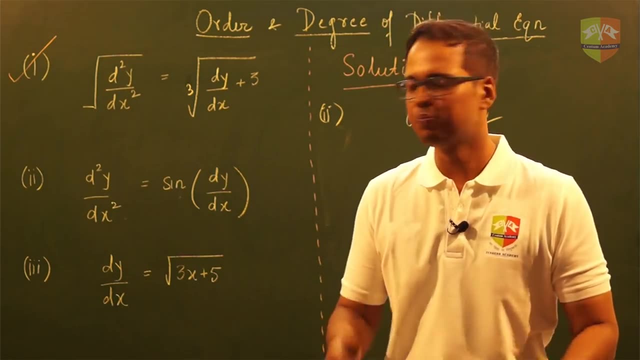 So x, and those powers must be whole numbers. So there is no sign term, there is no log term, there is no exponential term, So as to say there is no transcendental functions involved in a polynomial. Now, here being one, I cannot say that this is in the polynomial form. but hold on, can? 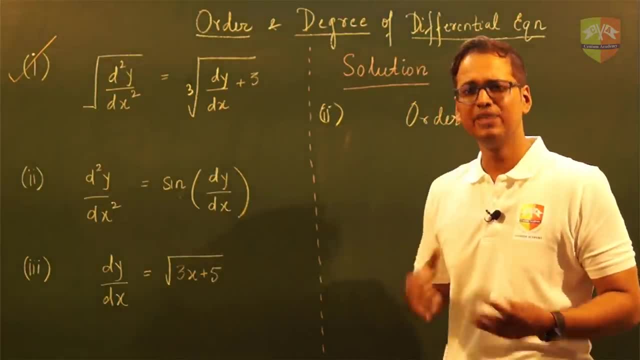 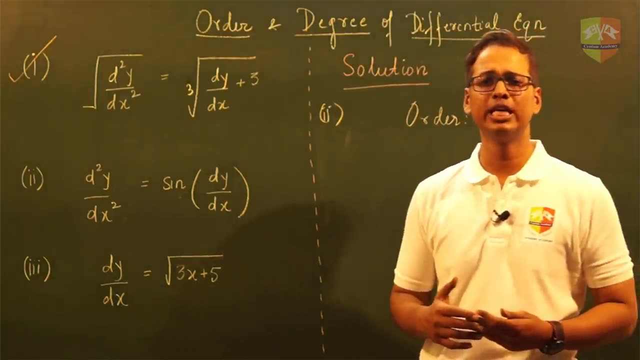 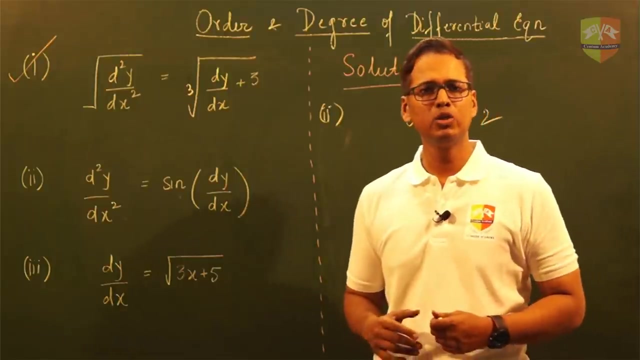 I get rid of it. if yes, then try to. if not, then we cannot find the degree for this particular differential equation right. or we say the degree for this differential equation is not defined Right Now. in this case, no matter how much ever we try, we will not be able to eliminate the 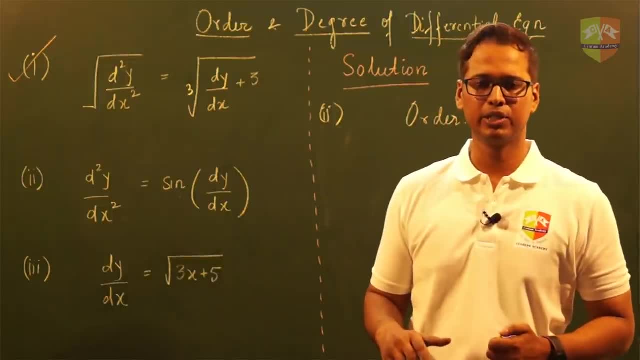 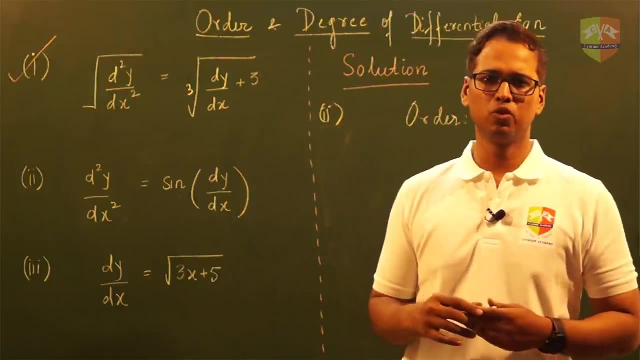 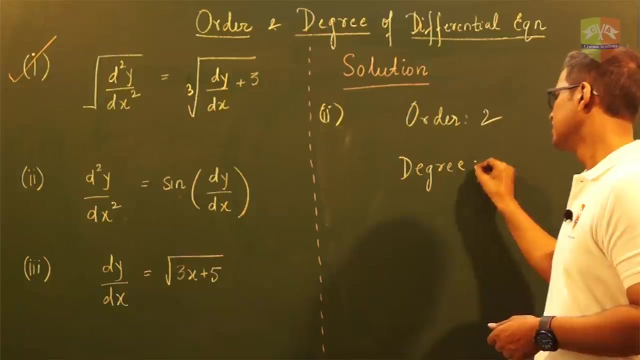 sign form from this particular differential equation, or in other words, we will not be able to convert this to a polynomial form in the all differential coefficients. So hence, for this particular differential equation, degree will not be defined. So we say degree is not defined. Okay, 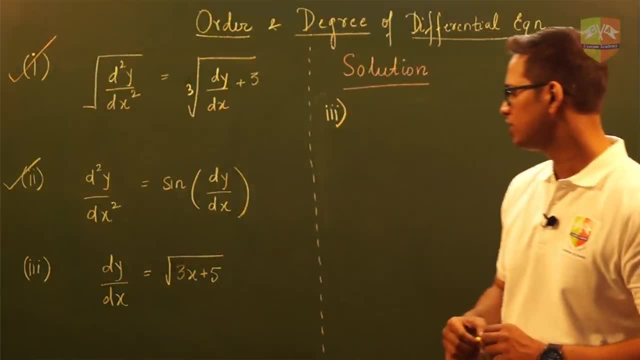 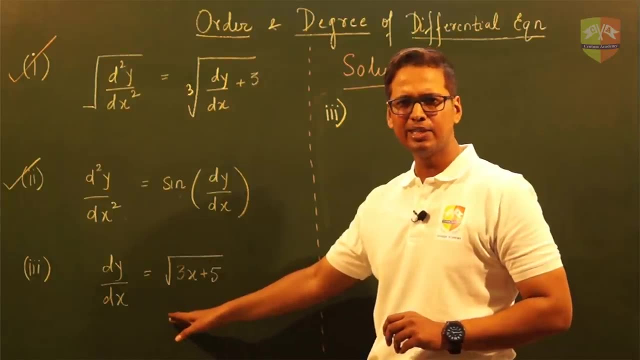 All right. So, students, coming to the last question, the third question, in this case, again, we have to find the order and the degree of this differential equation. order, again, is very simple. activity: we see only dy by dx. that is the only differential coefficient existing in this problem. 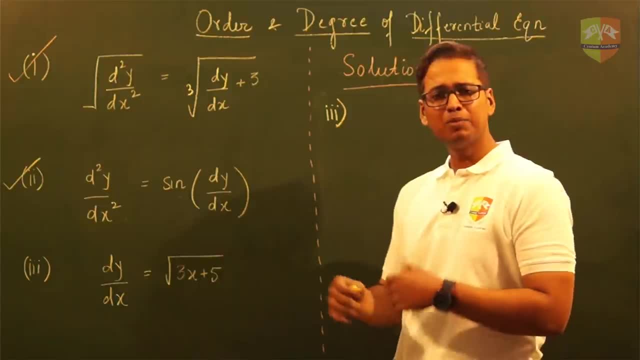 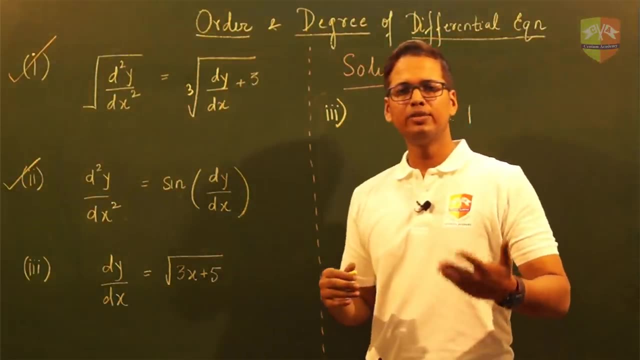 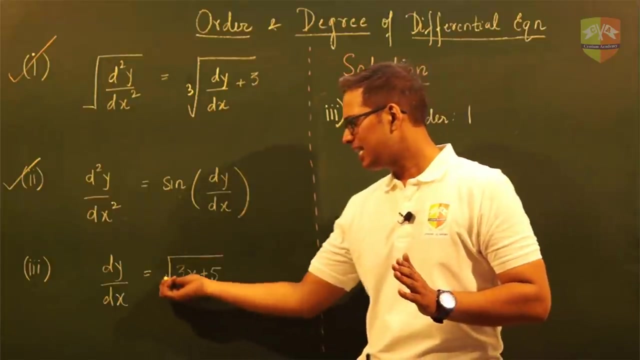 So it's an order one differential equation, right Now. what about degree? So order is one. What about degree? Now for degree, as I told you, we need to convert it into a polynomial of differential coefficients. Now many students get confused. They say that it is not a polynomial. 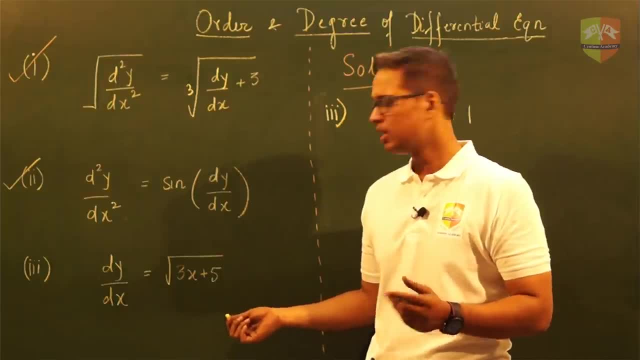 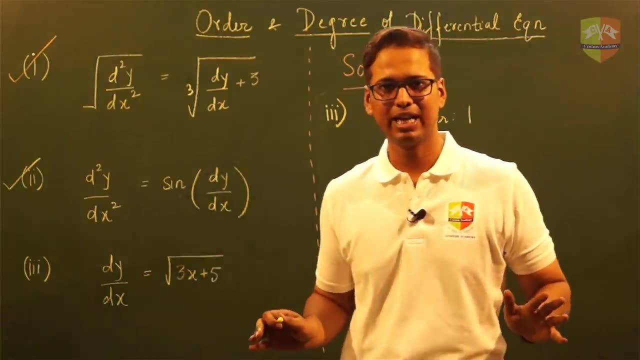 It is not in the polynomial form, So how are you finding the degree for it Now? please note: the under root sign on the independent and dependent variables are allowed Right. So in this case we have an under root on 3x plus 5.. 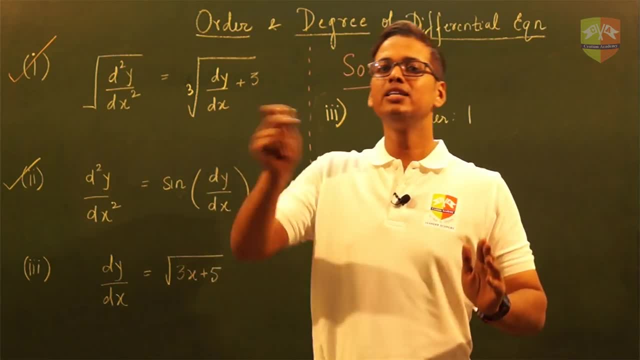 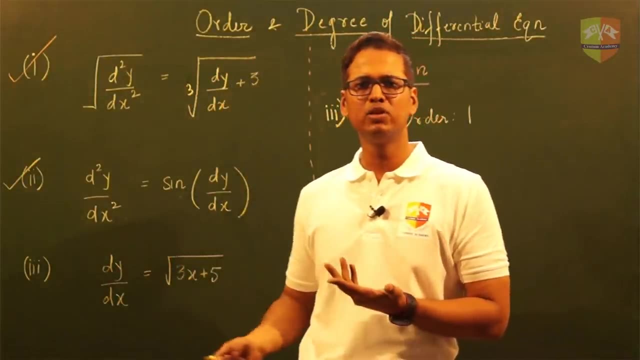 It does not involve any differential coefficient. had the under root been on some differential coefficient- let's say the root have been on dy by dx or some negative powers would have been on dy by dx Or a non whole number power should be on dy by dx then in that case, yes, I understand.